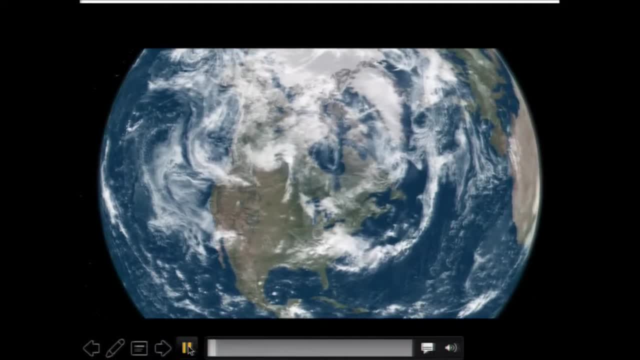 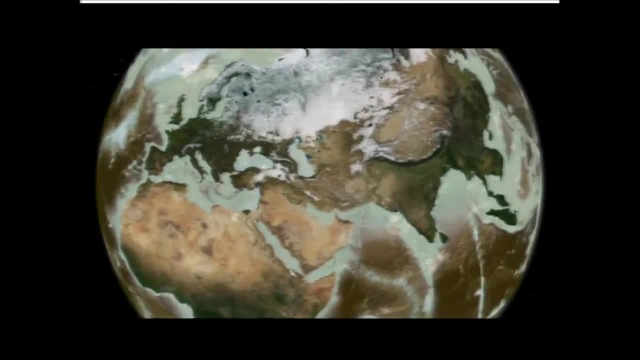 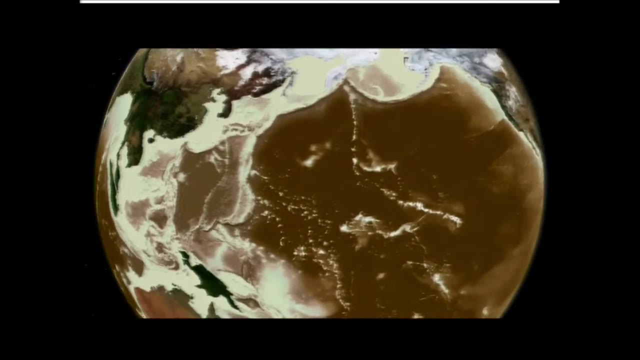 and see the wide expanse of seafloor sediments that cover again 70% of the Earth's surface. So we would see a range of compositions. We would see that snow line that Bernie talked about on ocean ridges And we'd see changes as we come up on the margins. 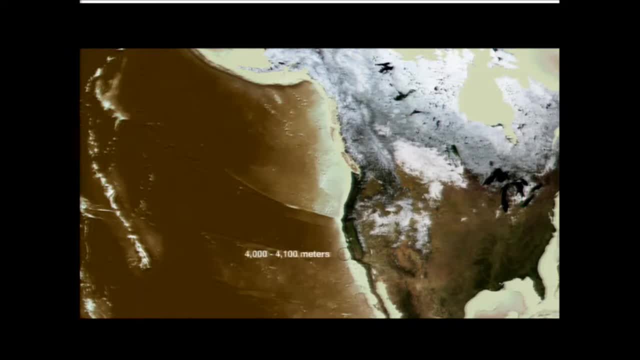 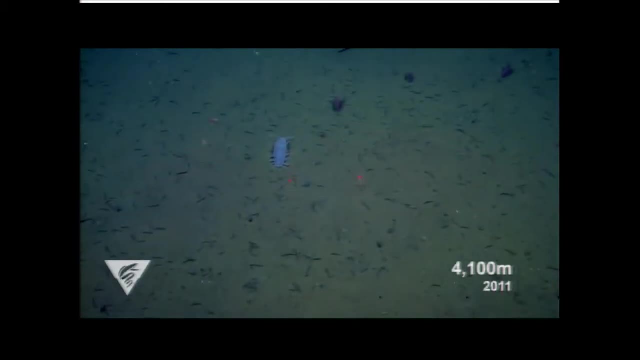 But what does the seafloor really look like? We've only learned that in recent years by using camera systems and ROVs, And most of what we learned before that about the seafloor was from sediment cores. Here's a little video showing you the seafloor. This is from a Bissell station, Station M. 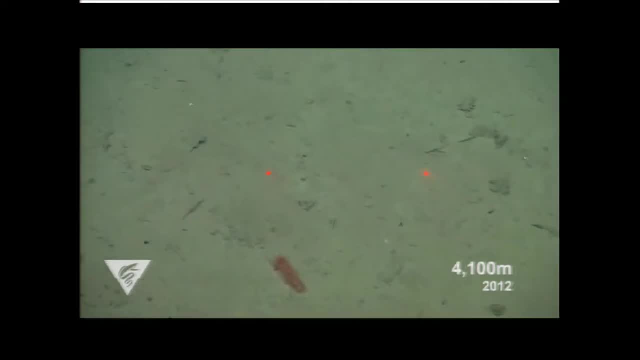 which Ken Smith at MBARI has studied for over 30 years. looking at the seasonality of fluxes in deep sea, You can see hemipelagic sediments, rich marine life, a lot of holothurians and fecal casts and that sort of thing. You know again, a lot of spatial variability, even in this deep. 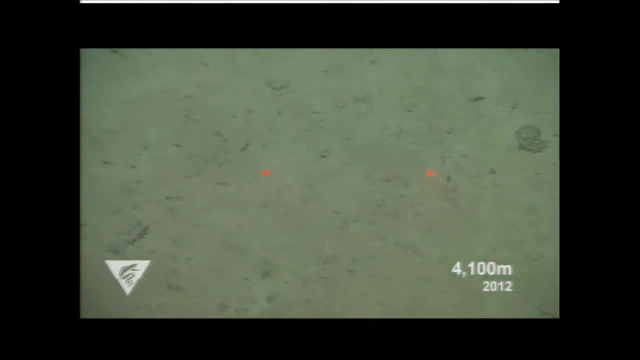 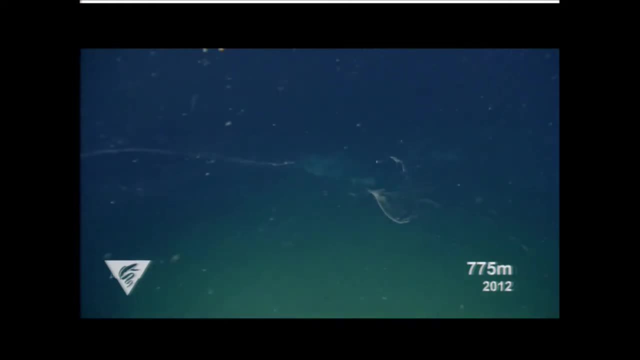 part of the ocean. The video here is going to transition now to another area I've been interested in, called Hydrate Ridge, off the Oregon coast. Notice the rain of particulate matter that comes to the seafloor, The constantination to be very near a productive margin. 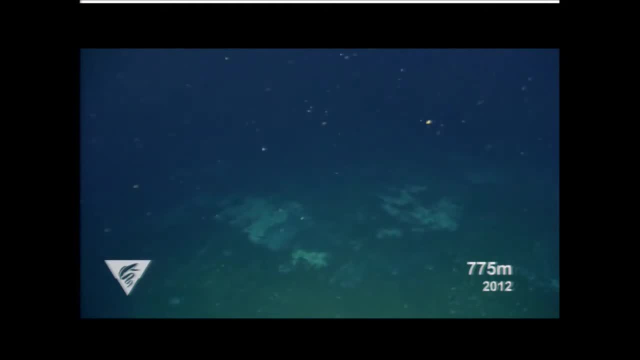 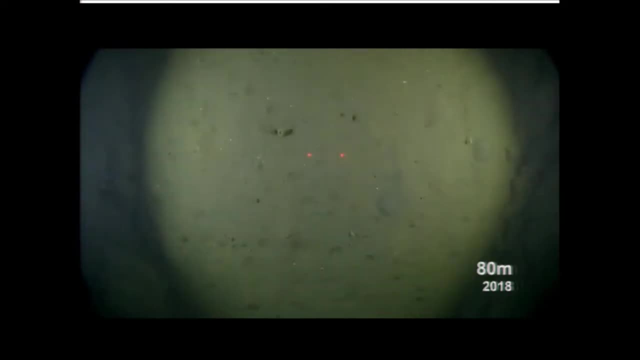 And we find chemosynthetic communities on the seafloor. These are some bacterial mats forming over an area where there are gas hydrates just below the sea surface. Or we can move on to the shelf where we've been studying- the Oregon shelf. 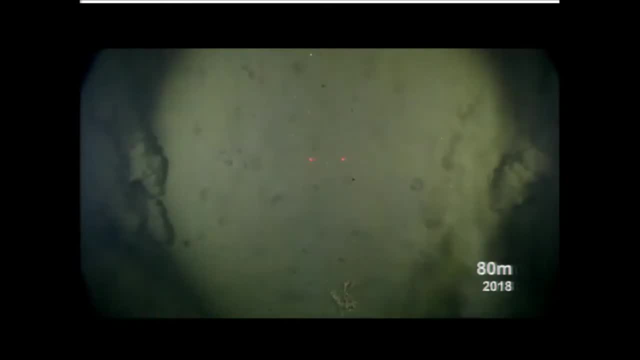 We have sandy sediments. This is at 80 meters depth, Still highly bioturbated. In winter months, when you have storms, you see sand ripples Again. there's an extreme amount of information involved. It's been a pleasure to be here. 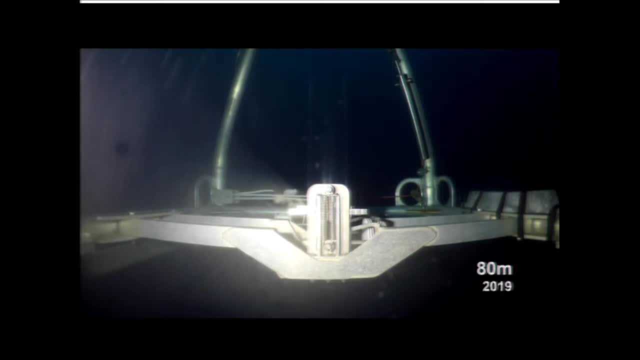 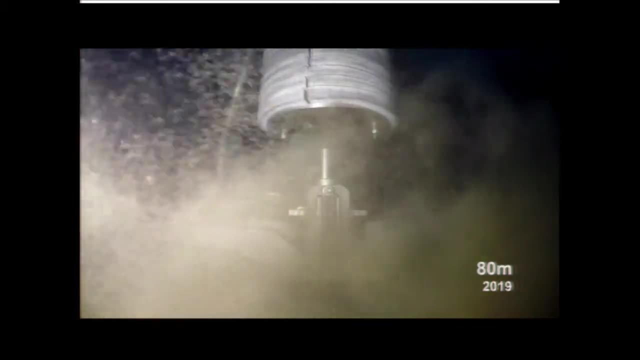 Thank you. wide variety of habitats and sediment types on the seafloor and, again, most of what we know about the seafloor comes from taking sediment cores. you ever wondered what happens when you send one of those things to the seafloor? here's. 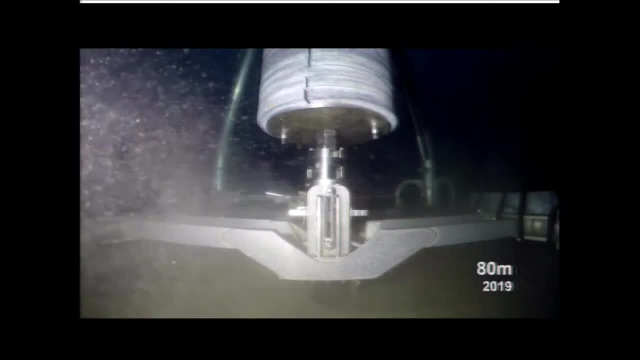 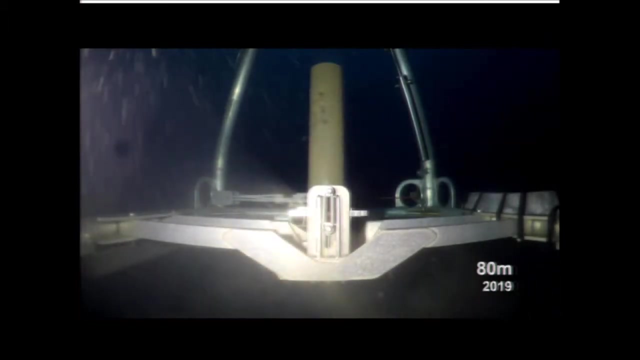 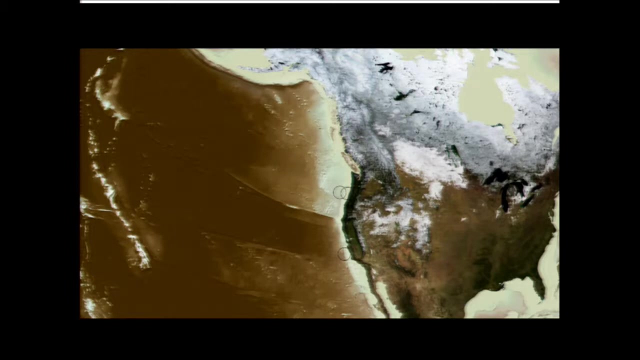 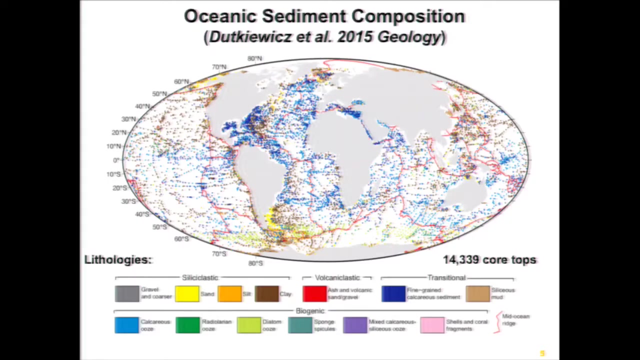 just a video using a system that we use for our studies on the Oregon shelf. it takes a essentially a gravity core that pulls up a nice about 50 centimeter sand core that we bring back for characterization and core incubation again. so that was just to try to get you enthusiastic about the seafloor now. 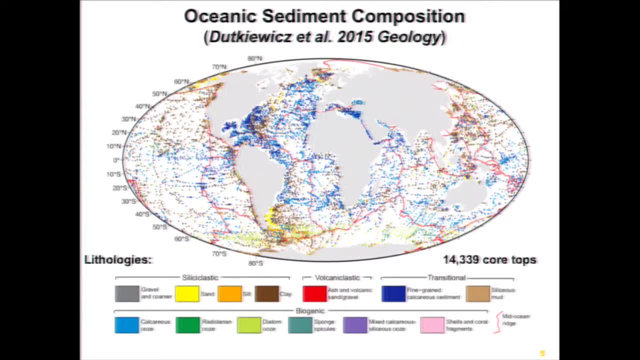 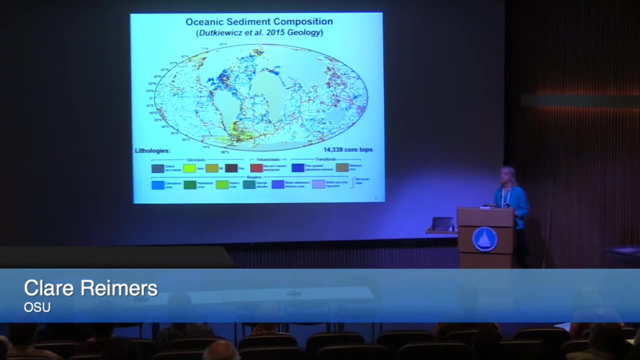 again. I mentioned most of what we know about sea floor biogeochemistry has come from collecting sediment cores and having archives of these cores, and this is a figure from a nice paper that was published in geology in 2015 showing the the lithologies of surface sediments. 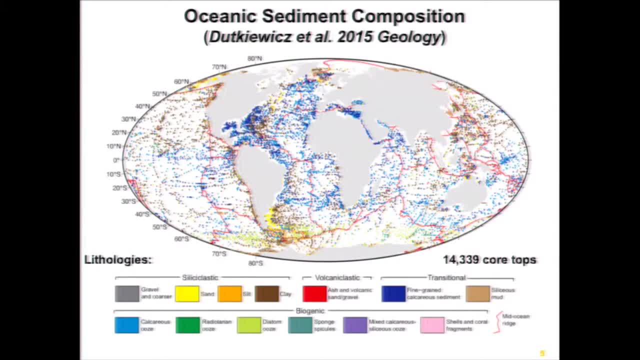 globally, based on over 14,000 core samples and the. the authors of this paper, who are from the University of Sydney in in Australia, make a nice point that the the surface distributions of lithologies and compositions and accumulation rates of sediments, really helps us understand. it gives us an underpinning for understanding ocean. 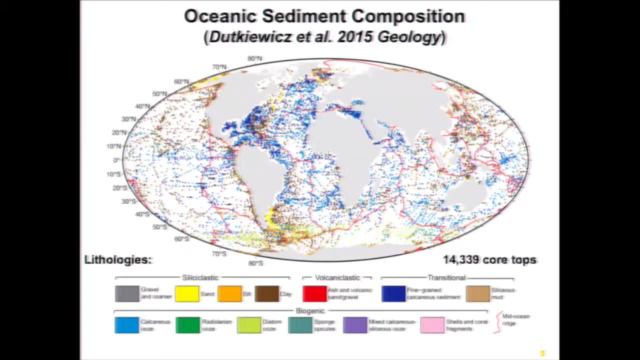 biogeochemical cycles and sediment transport in the ocean. of course, cores. Those are also our window into the past, through downcore studies of the Paleoceanographic record and past patterns of ocean primary production. In this figure, for instance, you can see, if you look at the blue colors, the calcareous, 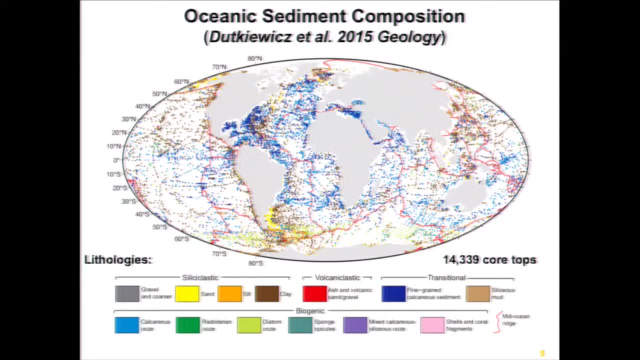 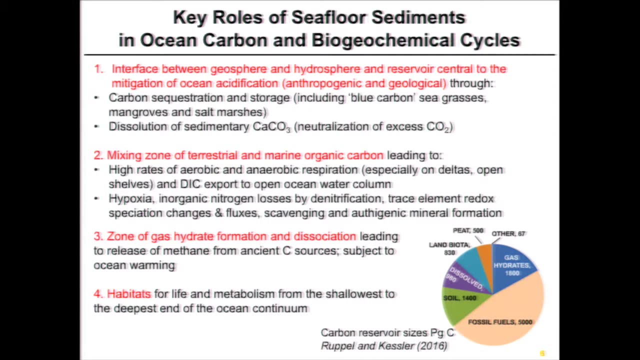 oozes that again are on the ocean, ridges along the equatorial Pacific, large parts of the Indian Ocean, and then the siliceous oozes that ring, for instance, the Southern Ocean. So in this session again we're going to cover a number of habitats, but there's some. 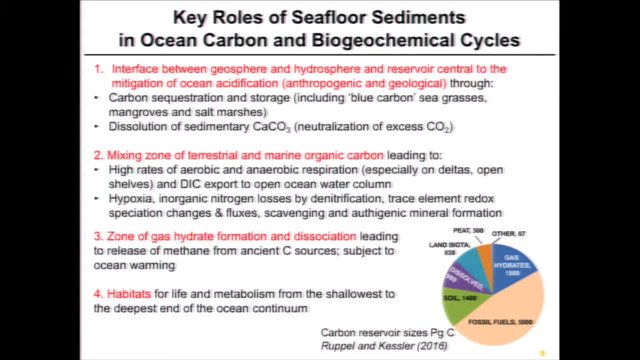 key points that we'd like to stress about the roles of seafloor sediments in biogeochemical cycles. The first is that this interface is, you know, a geochemical interface, An interface between the geosphere and the hydrosphere, and it's a reservoir. that's central. 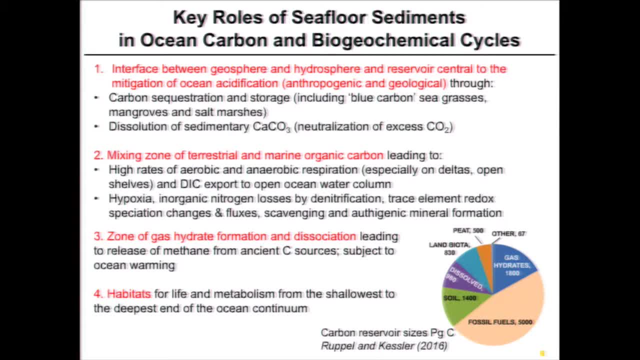 to the mitigation of ocean acidification. We heard about that in this morning's session and you know that's particularly through dissolution of sedimentary calcium carbonate. But our, as Tom Bianchi reminded us yesterday, sediments particularly on margins and in. 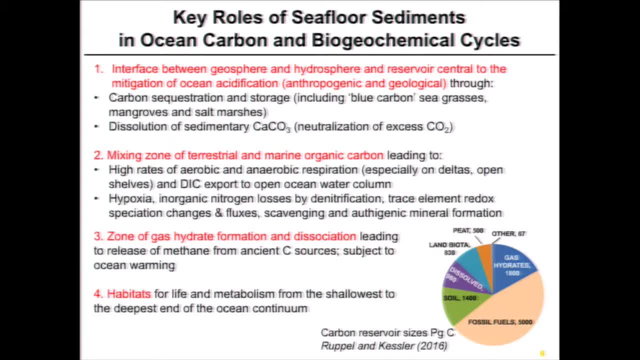 areas like deltas are where, or fjords are areas where there's carbon sequestration through burial Sediments. seafloor is also a mixing zone for terrestrial and marine organic carbon, and this can lead to high rates of both aerobic and anaerobic respiration. 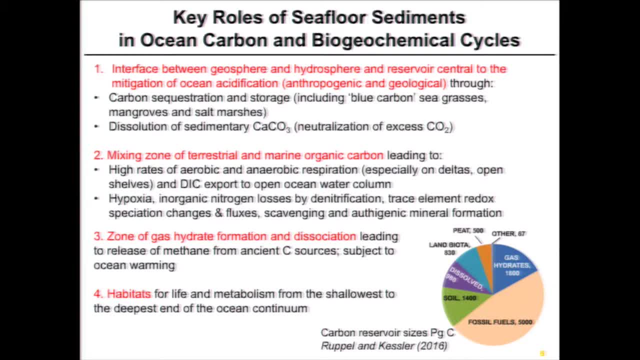 And this can then lead to the return of the IC to the water column and its export to the open ocean from margins. In our first session of this meeting, we heard about ocean deoxygenation and hydrogenation, So we're going to talk about that. 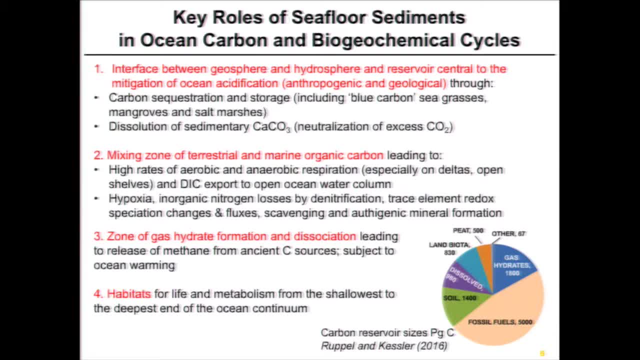 Hydrogenation and hypoxia. hypoxic areas are tied to these areas of high respiration, And these are also areas, of course, where we have inorganic nitrogen losses by denitrification, trace metal, redox, speciation changes and fluxes scavenging and othogenic mineral formation. 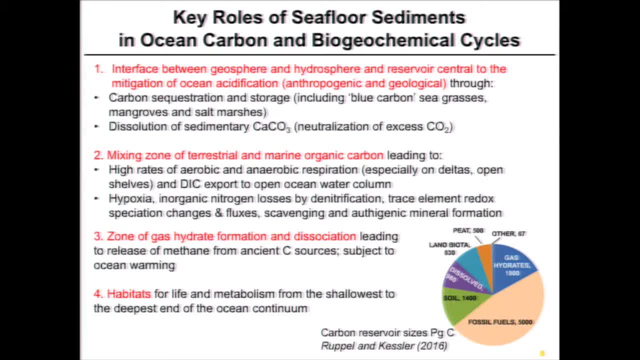 Another reason to think about the seafloor is this is a zone of gas hydrate formation and disassociation. Thank you, And Katie will be talking about this process in the Arctic. And then, of course, last but not least, seafloor is a vast habitat for life and for 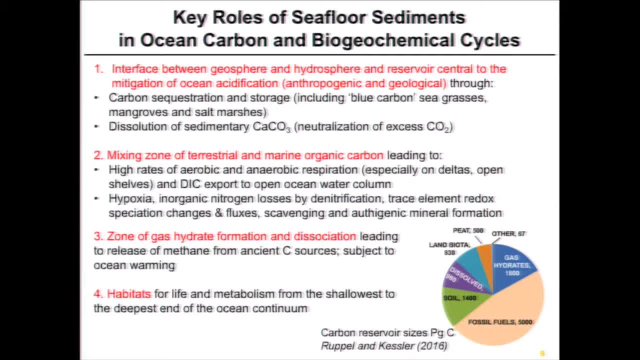 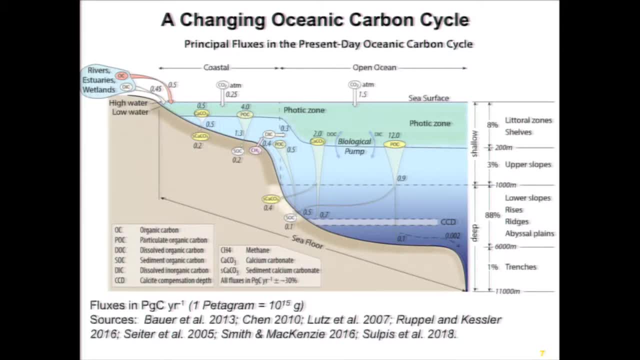 metabolism, and it spans, of course, from the shallowest depths to the deepest depths of the ocean continuum. So in preparing for this session, I put together this figure. It's to try to compile, Okay, Okay So, in this figure the role and sort of the relative magnitudes of fluxes to the seafloor. 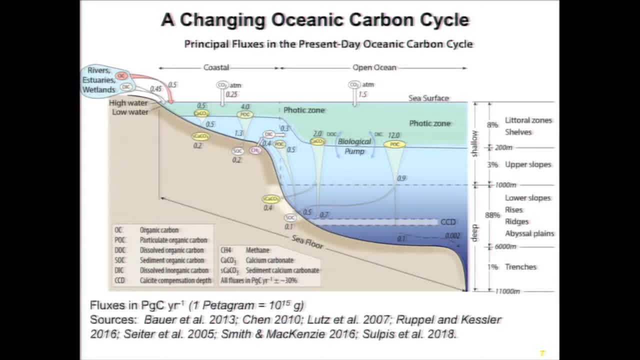 in the carbon cycle compared to other parts of the carbon cycle, And we can debate a lot the numbers, but I want you to sort of look at some of the relative magnitudes, And this is based on what's considered the present-day oceanic carbon cycle. 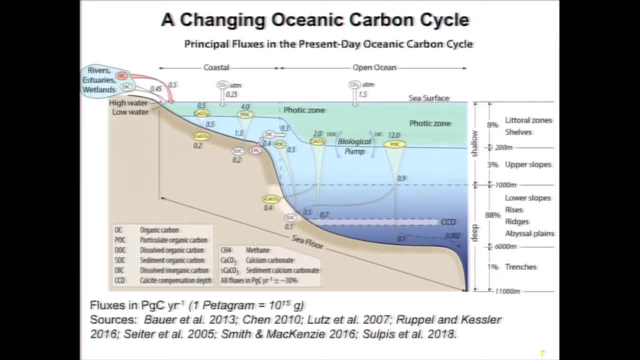 So by present-day, you can see in this figure that the CO2 flux- I've got a little bit more time, I've got a little bit more time- Okay, The net flux into the ocean from the atmosphere is well, it is into the ocean in both the coastal and the open ocean areas. 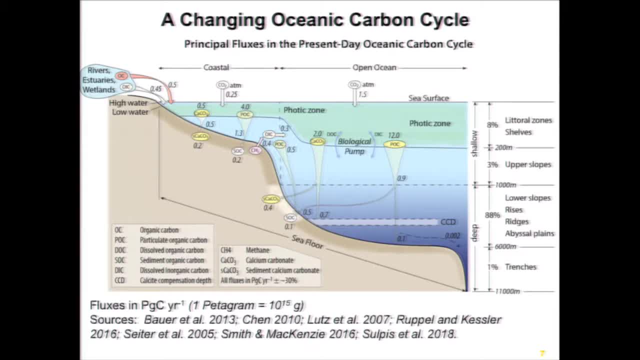 It's portrayed that way, But I've also tried to highlight fluxes to the seafloor and tried to separate again the sort of upper part of the ocean above 1,000 meters- So 1,000 meters- and the deep ocean. 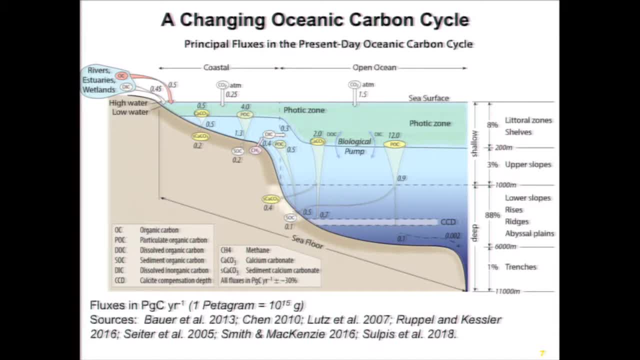 And one of the reasons for that is that when carbon reaches the deep ocean, either if it's buried or even remineralized in this zone, at least it's sequestered from the atmosphere on human time scales. So we are interested in what fluxes do come down through the biological pump to this realm. 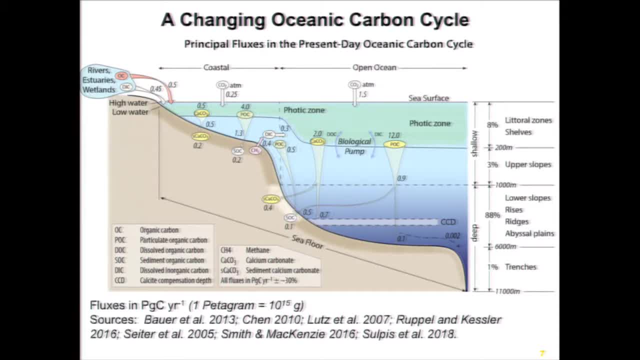 And so what I wanted to walk you through now is just how we have some estimates for the magnitudes of those fluxes. Will Berrelson said, I think, at one point: how do you put a number on some of these things? 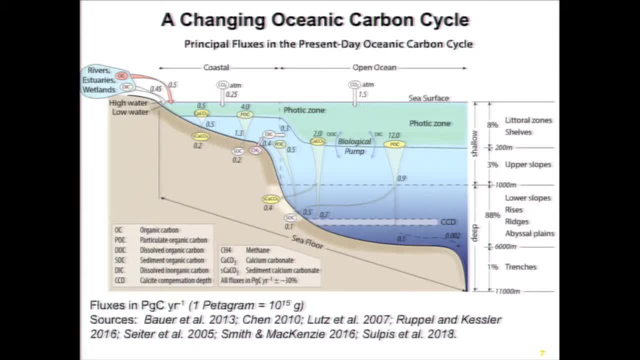 So I want to show you how we put one number on this figure. It's the carbon flux to the seafloor below 1,000 meters, And I'm talking now about the organic carbon flux. And just a reminder, I'm talking about 88% of the ocean when I talk about the seafloor below 1,000 meters. 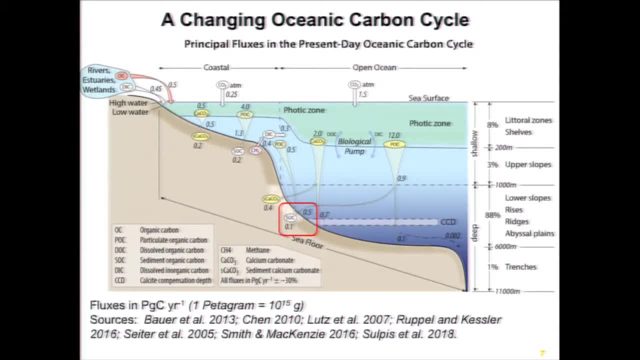 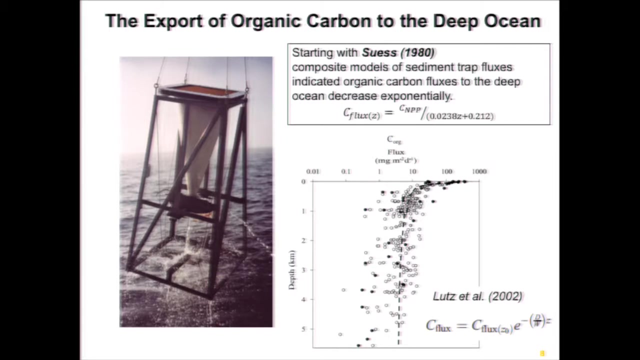 So how have we come to know the magnitude of this flux, which again is a carbon flux, that is, again removing carbon from immediate contact with the atmosphere? Well, our first estimates of this flux really stem from programs that started in the 1970s, where sediment traps were put out globally. 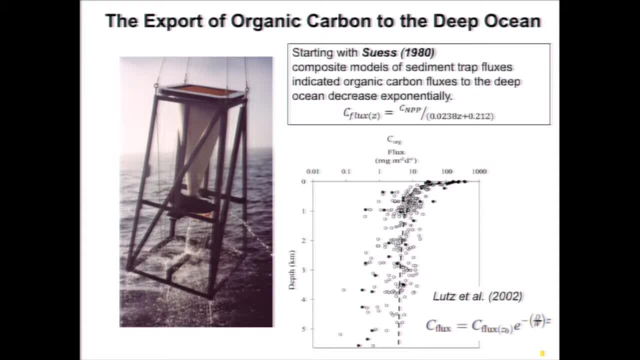 to measure the sinking flux shown here in this diagram as milligrams per meter squared per day, as a function of depth. The very first compilation of such sediment traps fluxes was made by Erwin Seuss, who happened to be my thesis advisor. 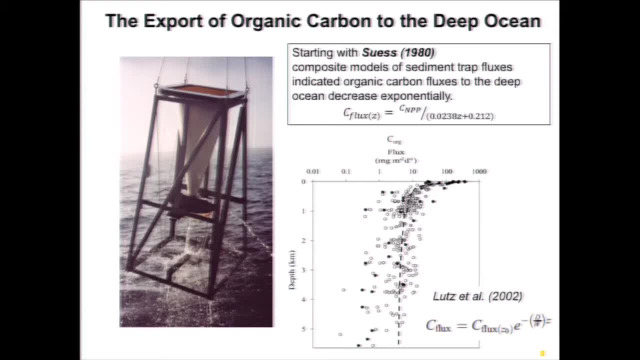 That's why this one was drilled into me, I guess you might say- But the observation that there was an exponential decrease in carbon flux with depth in the ocean, but that it scaled with the net primary production at the surface. The Seuss relationship was based on the data that's shown. 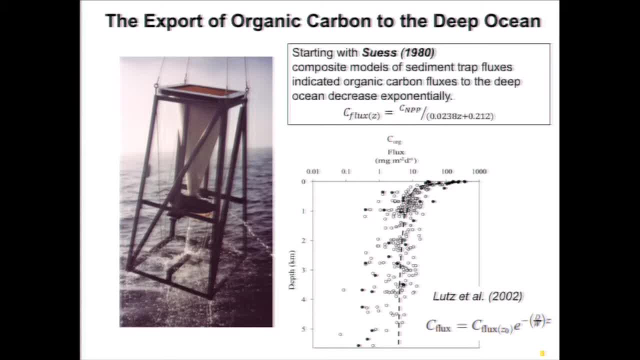 it included the solid symbols in this diagram, which is from a later paper by Lutz et al. Of course, there's been a lot more data that's been added, and a lot in this figure came from the Jay-Golfs program, and so we had revisions of these exponentially decreasing relationships. 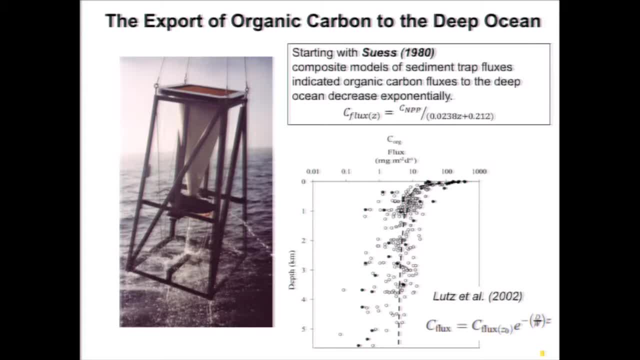 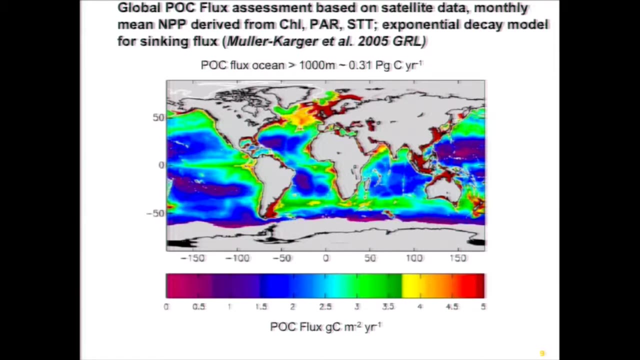 but the systems can still bear fruit, right? Uh-huh, Uh-huh. the general model stays the same, and the thought that carbon drops off as a function of depth and degradation rate and settling rate of particulates. So just to remind you, then, that this kind of relationship was used by Mueller and Karger. 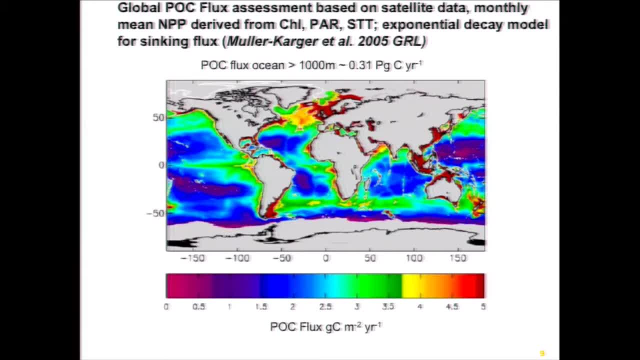 et al in 2005,, combined with assessments of net primary production, that's based on satellite information and models of chlorophyll, PAR and sea surface temperature, and also then ocean bathymetry, to come up with, again based on the sinking flux, a global distribution. 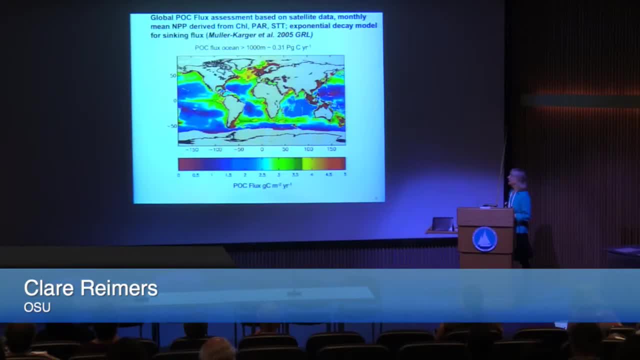 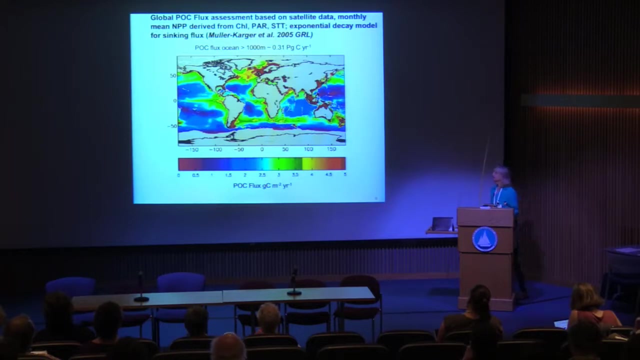 for the POC flux to the seafloor And if you integrate this figure which they produced for the areas of the ocean below 1,000 meters, the global flux is 0.31 petagrams of carbon per year And for the margins they get about twice that, or 0.6 petagrams of carbon per year. 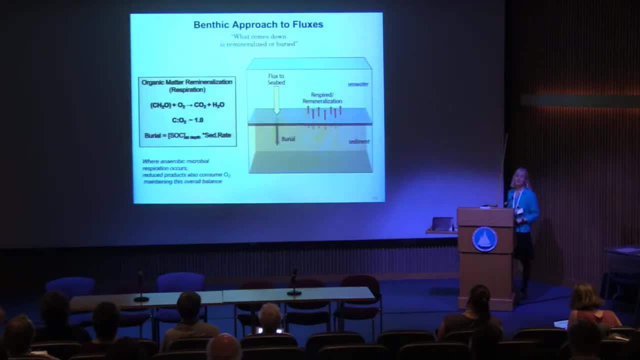 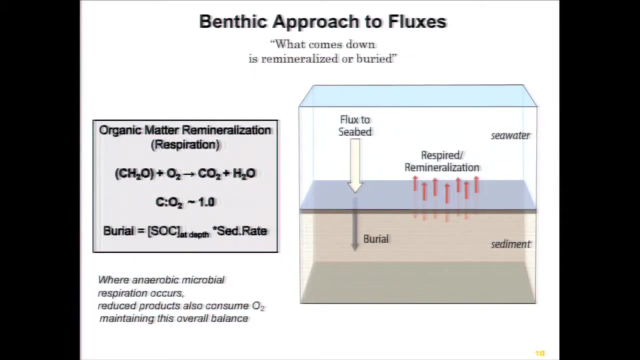 Well, there's another approach to carbon fluxes which gives us a slightly different answer, and that's based on localization. So it's important to look at the seafloor, because the seafloor is our ultimate sediment trap, And one advantage of the seafloor is that, unlike sediment traps, you're going to see- 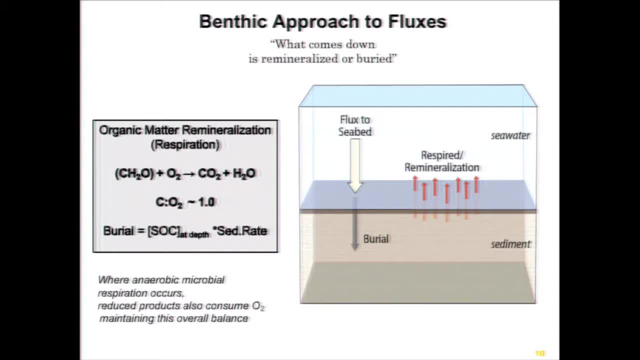 lateral inputs, particularly near the margins, and sediment traps may miss those inputs. So again, the idea to assess flux to the seafloor, and it could be for carbon or silica or any part of the biogeo-capital cycles. Is it an area of a carbon? YES, 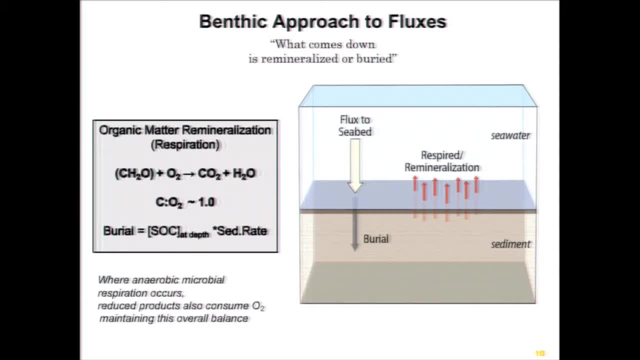 is that the flux to the seabed has to be equal to the sum of what is remineralized and what gets buried. And in the case of organic carbon in the deep ocean, almost all of the flux is remineralized. So if we measure that remineralization rate, 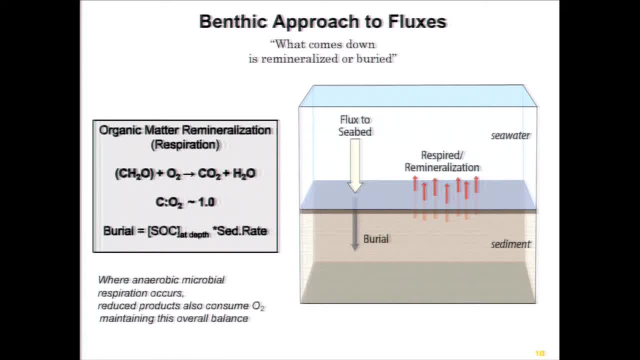 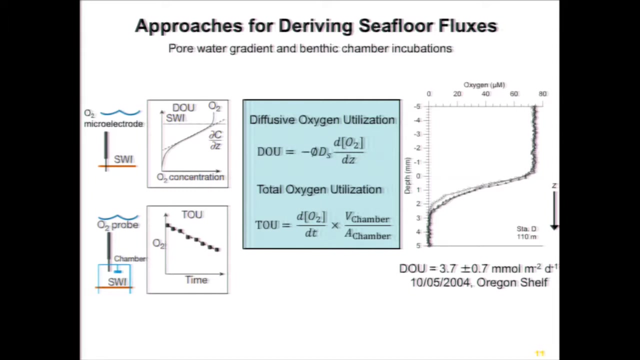 we have a good measure of the carbon flux to the seafloor, And so one approach to that is to measure the oxygen flux, because in the deep ocean most of carbon is oxidized through aerobic respiration, So we use oxygen fluxes as a proxy for carbon fluxes. 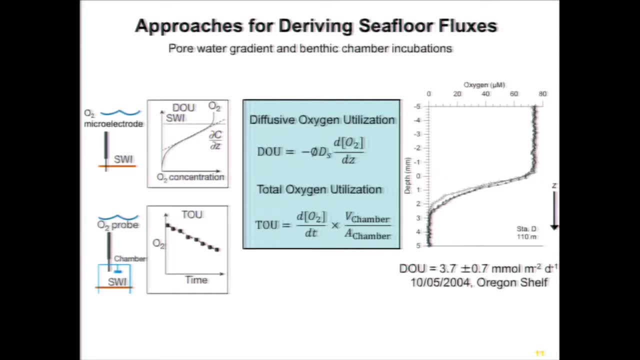 Briefly, until recently, there were two main methods for arriving at oxygen fluxes, And again these developed in the last few decades. The first is based on modeling pore water gradients And in case of oxygen, we were able to measure highly resolved 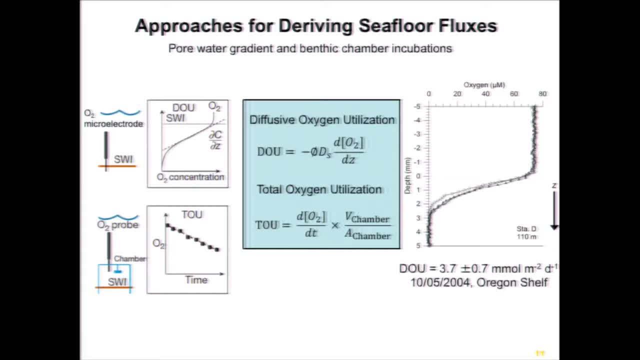 pore water gradients using microelectrode sensors that can be deployed in situ to measure gradients across the sediment water interface. Here's an example from some of my work off Oregon showing oxygen gradients profiles that only extend a few millimeters into the sediments on the Oregon. 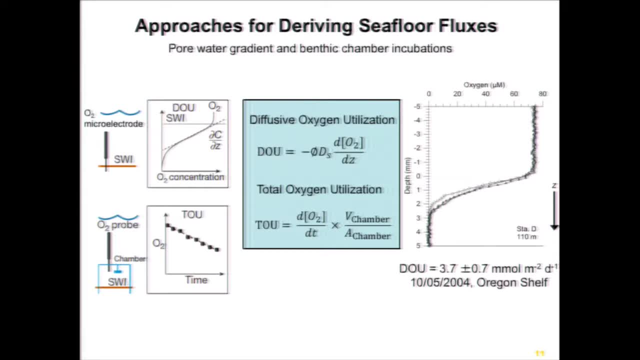 shelf. But again, based on that change of oxygen and the assumption that the transport of oxygen into the bed is dominated by molecular diffusion fluxes, can be calculated as diffusive oxygen utilization rates, or DOU, The other approach again, which can be done in situ. 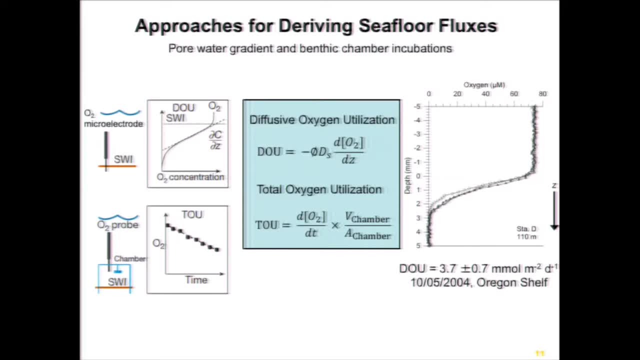 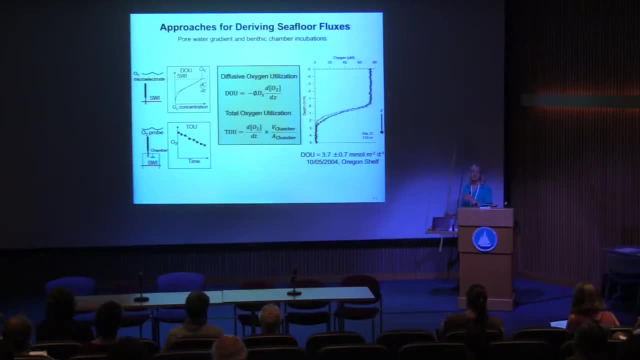 is to put a benthic chamber over the seafloor, enclose an area of the seafloor, incubate it and absorb it And observe the uptake of oxygen or the release of CO2, or the release of nutrients. 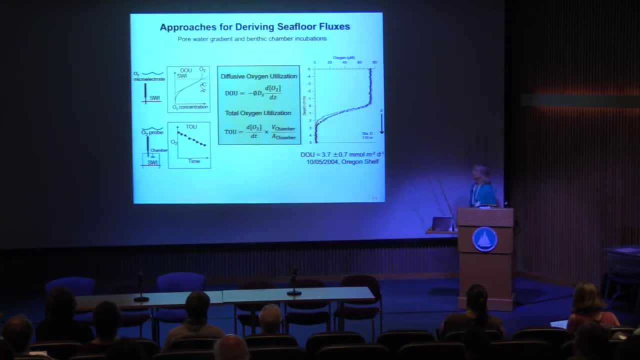 And this is another technique. It does not assume that the only transport mechanism is molecular diffusion. so it's termed the total oxygen utilization And generally we see in the coastal ocean total oxygen utilization rates do exceed diffusive oxygen utilization rates because 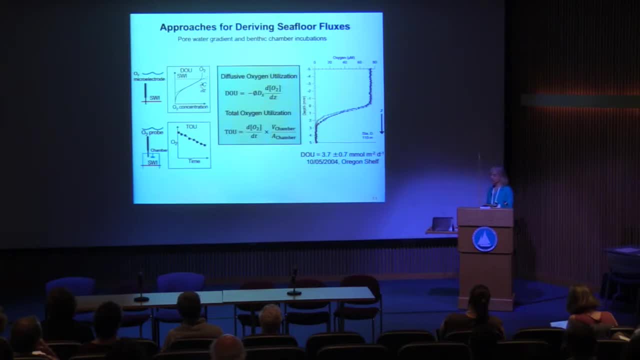 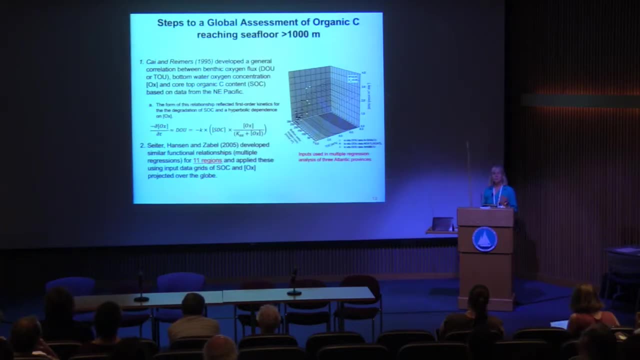 of the influence of biotrapeutes, DR PETER SALGO, DR CATHY L MAHER, in bio irrigation. okay, I'm running out of time quickly. so the way we got to a global estimate was to. this was recognized by Weijun Cai and myself that 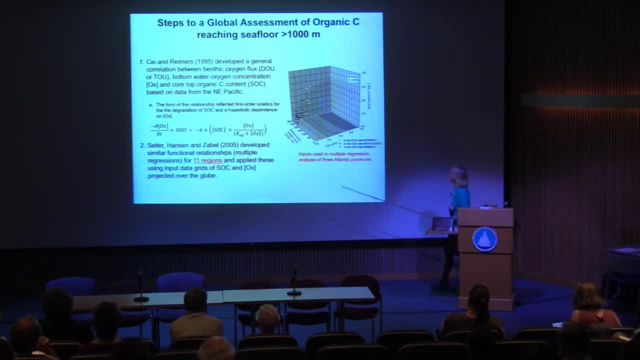 there seemed to be a relationship between dou and sediment, organic carbon and bottom water oxygen- you know the the two reactants, carbon and oxygen- and and so one could form empirical relationships between these, these parameters. we developed one, first for the Northeast Pacific, and then, following work by Sider et al, based on a lot of later data, largely measured by. 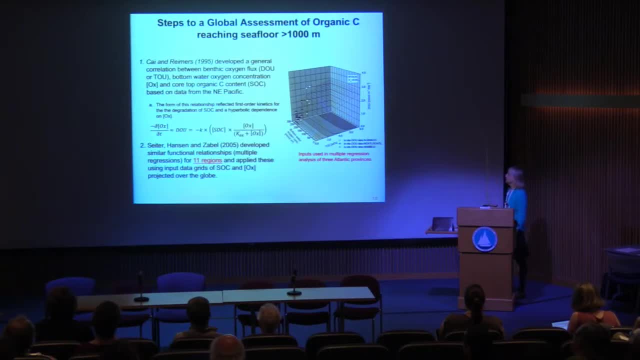 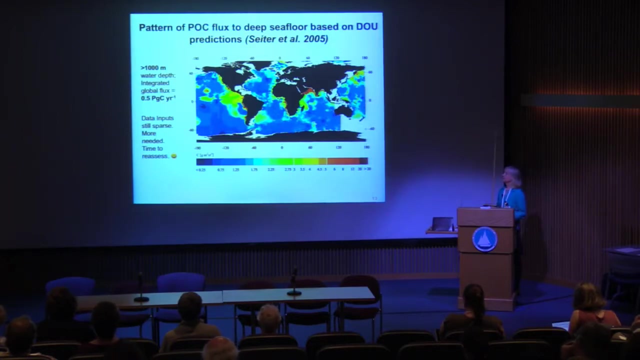 Ronnie Glud's group. they put together other empirical relationships, these multiple regressions for 11 regions, and and again came up with sort of global estimates of the particular organic carbon flux to the seafloor which again could be integrated to give us a global flux. it's 0.5 petagrams of carbon per year. I just 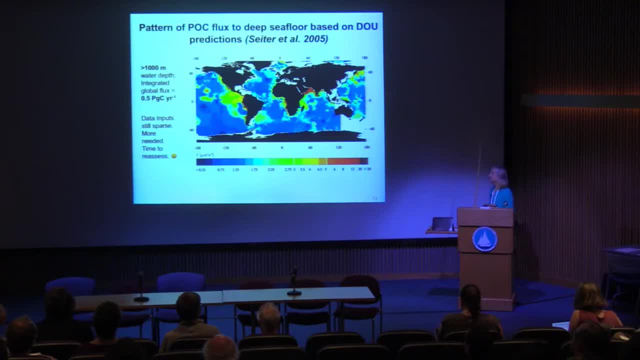 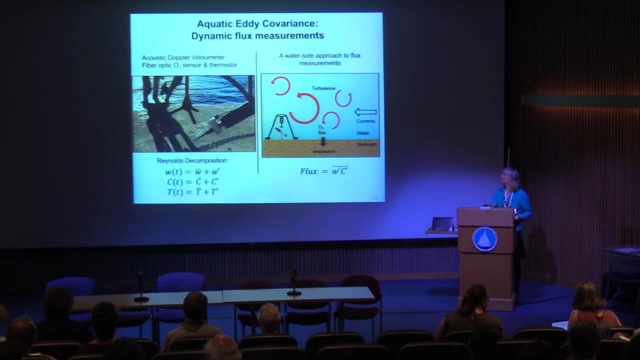 wanted to say that the data behind all this is still sparse. more is needed, and and one one question we can ask is is: are these fluxes changing, as we've heard that the, the biological pump, is changing, calcification rates are changing, so how is that reflected in fluxes to the seafloor? all right, so just a real quick. 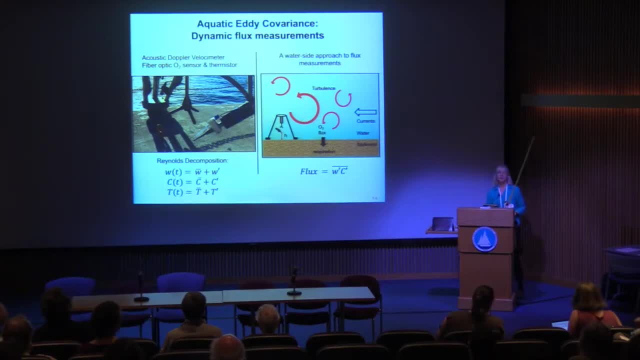 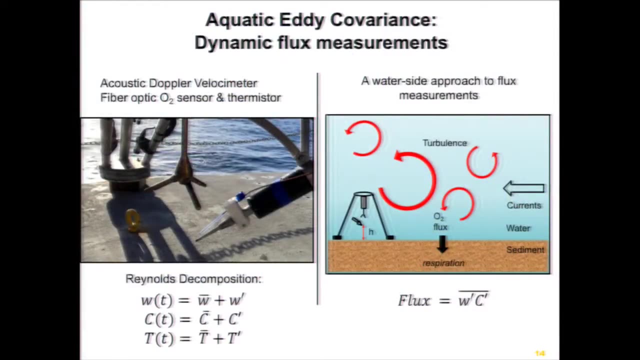 I guess I'm going to run out of time. any covariance is a new method for assessing benthic fluxes. it's being used primarily for measuring oxygen fluxes. it requires two sets of sensors: an acoustic Doppler velocimeter that measures velocities and, in case of oxygen, and some 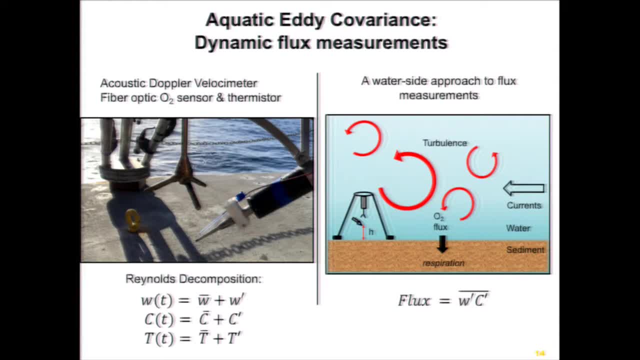 kind of oxygen sensor, and this picture shows a fiber optic oxygen sensor together with a thermistor. it's what we would call a waterside approach to flux measurements, because you're measuring velocities and oxygen usually about 15 to 30 centimeters above the bed in a rapid time series which then gets 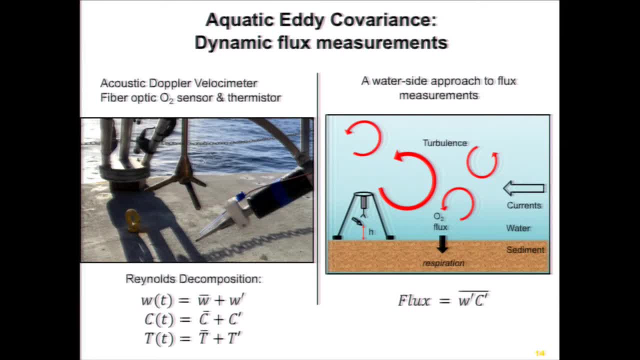 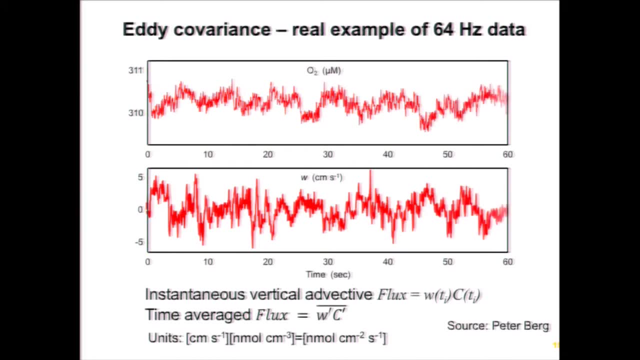 separated into average and varying variation components. so again, we make these measurements usually at 64 times a second, 64 Hertz. this is an example of 60 seconds of data, and this is what it might look like. but to gain, arrive at a flux, we have to take a few steps. we need to separate the 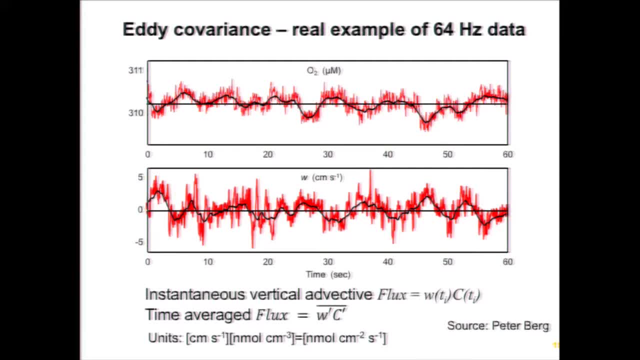 variations from a mean, and here there's just a short-term running average, put through the data to illustrate the separations from the mean. but what's key here is it just wants you to notice- is that there parts of the record, for instance, where the vertical velocity, that's W, is mostly towards the 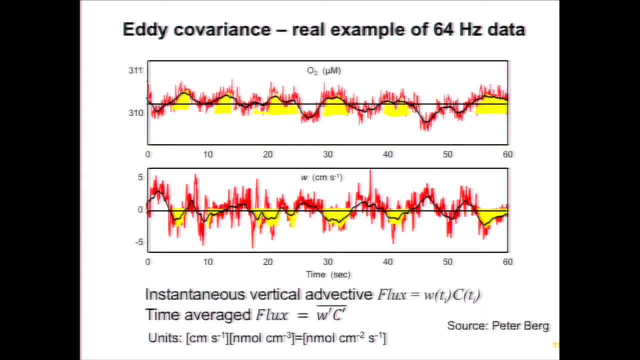 bed and in those periods of the record you tend to see higher oxygen concentrations, whereas other periods, when the velocity is away from the bed, you have higher oxygen concentrations. and this is a case where this- the bed- is an oxygen sink and what you're seeing is the effect of eddies passing by the sensors and eddies. 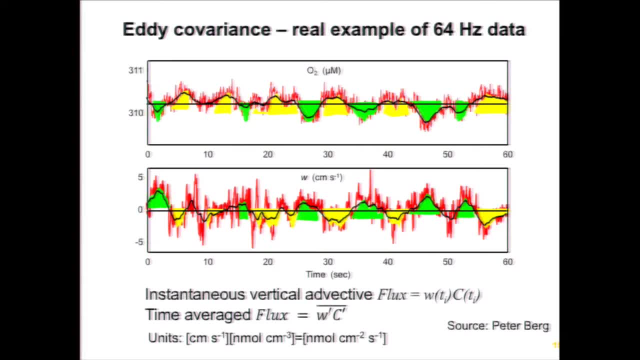 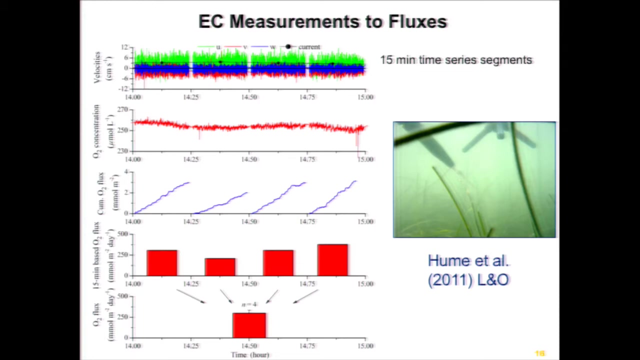 that have been in contact with the seafloor have a little less that those will. water parcels have a little less oxygen as they move up away from the bed than those that are moving down towards the bed, and so we take a time average of these variations to arrive at a flux, and, as you'll see in the next talk,